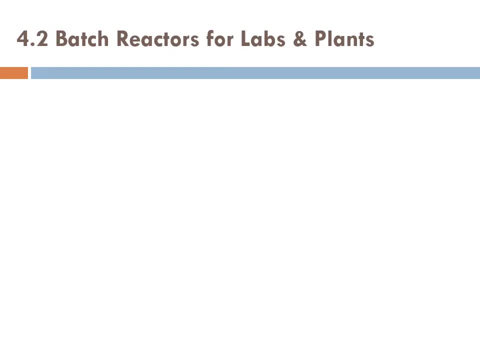 apply the five-step algorithm to the design of a batch reactor. One of the jobs in which chemical engineers are involved in is the scale-up of laboratory experiments to pilot plants, operation, demonstration scale or to full-scale production. Of course, whenever new technology is developed, first it is 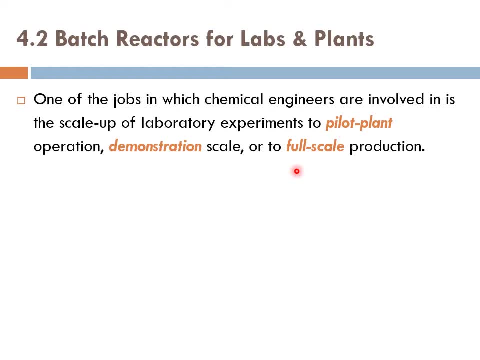 developed in the lab and then converted to the lab. So it is converted to pilot plant and then demonstration scale and finally to the full scale, meaning full scale production, meaning the plant, the actual plant. So it always, almost always, starts in a lab. In this section we discuss more about the 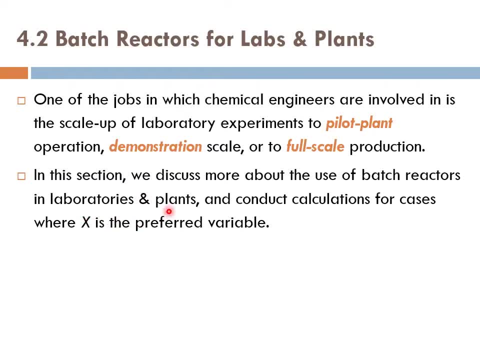 use of batch reactors in laboratories and plants and conduct calculations for cases where X is the preferred variable. Remember we are in part one of chapter four and in part one in chapter of chapter four we are interested in utilizing design equations written in terms of conversion. In part two of this, 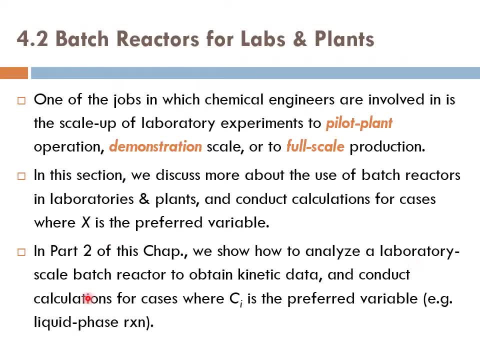 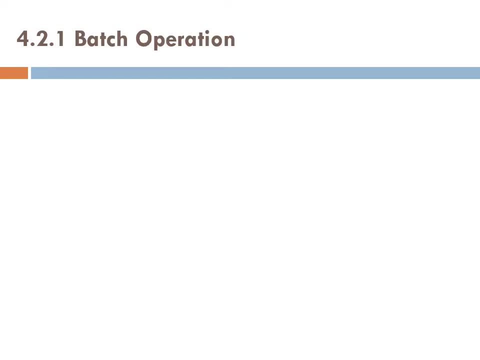 chapter we show how to analyze a laboratory scale batch reactor to obtain kinetic data and conduct calculations for cases where concentration is the preferred variable. Okay, so let's talk about batch operation. Batch reactors are usually analyzed with a constant volume assumption. and you know why? Because it's we're either using it. 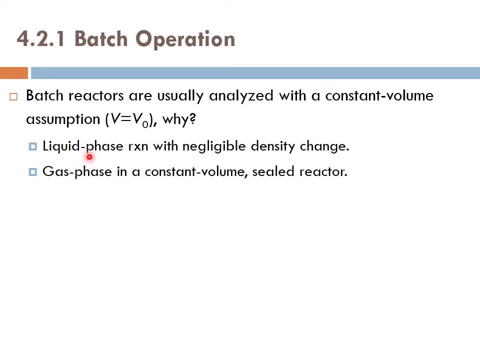 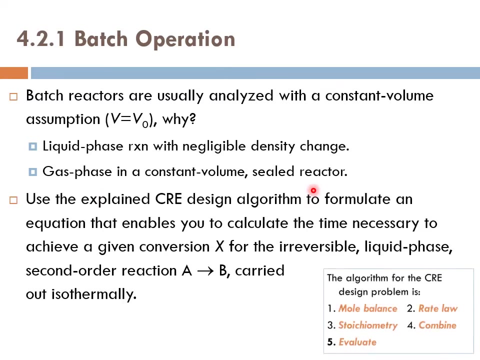 for liquid phase reaction, where you have negligible density change, or we use it for gas phase reaction, but the reaction is still constant. And the reaction is still constant carried out in a constant volume sealed reactor. Now use the explained CRE chemical reaction engineering design algorithm, the five-step algorithm, to 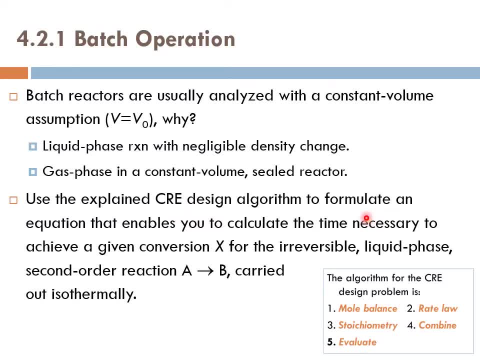 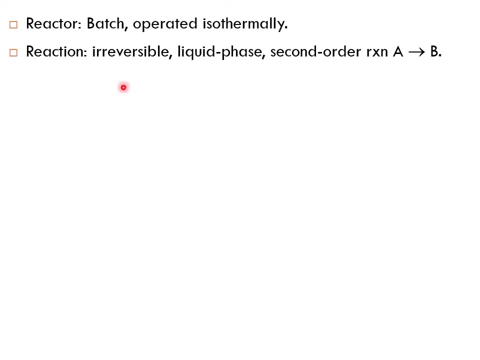 formulate an equation that enables you to calculate the time necessary to achieve a given conversion: X for the irreversible liquid phase. second order reaction A goes to B, carried out isothermally. So let's do this together. remember, the reactor was a batch reactor, operated isothermally, and the 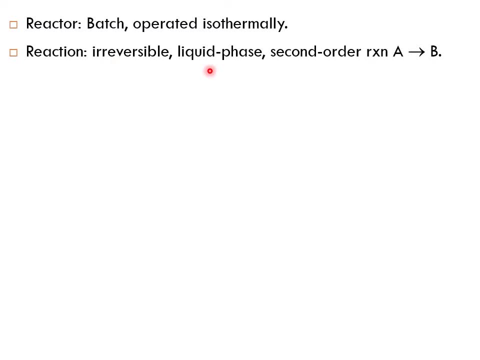 reaction was: irreversible reaction. liquid phase. second order reaction: A goes to B- Okay, so we want to design the CRE problem, meaning that we need to calculate the time necessary to achieve a given conversion. X for the irreversible liquid phase. second order reaction: A goes to B- okay, so we want to design the CRE problem, meaning that we need to. 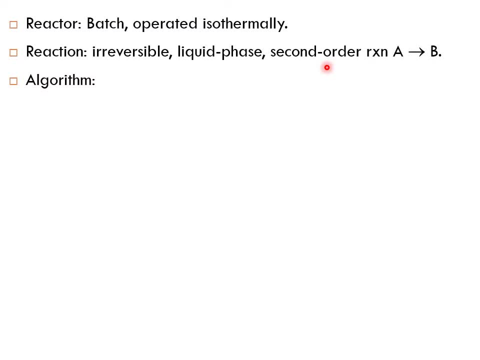 find the time because it's a batch reactor. so when we design a batch reactor, we're interested in finding the time, the required time, to achieve a given conversion. of course, the first step was the mole balance. so we select the correct mole balance and this is the mole balance for a batch reactor and A. 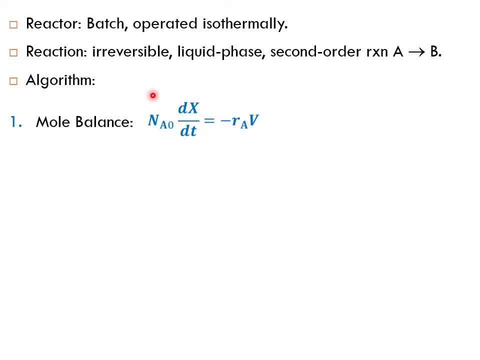 naught times DX over DT equals minus RA times V. then we go to the second step, which is the rate. we go to the second step, which is the rate low- see Shabab. here again, this is the most important equation in the design algorithm, because this is this is the 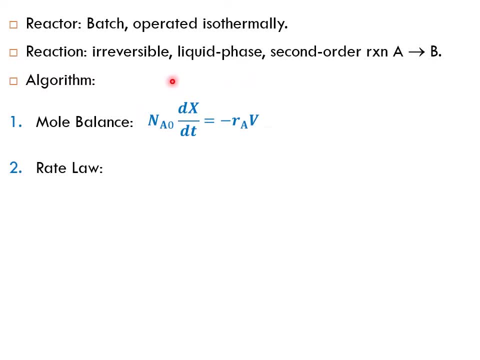 rate low- see Shabab. here again, this is the equation which it will enable us to find the required time to achieve a given conversion. however, when we wrote this equation, we actually introduced a variable: the rate of reaction. you know that the rate of fraction changes with time. it's a variable, so we need to provide an equation for. 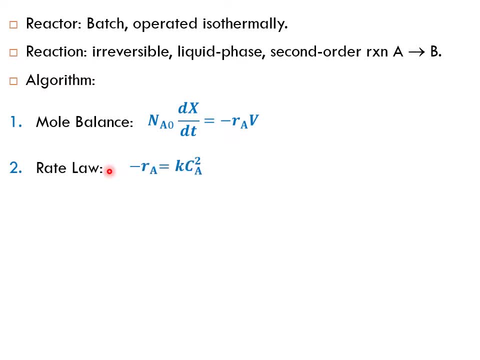 um. this equation is known as the rate law. so here we go. the rate law is written as: minus r a equals k times c a to the power 2, since we have a second order reaction. okay, now that we provided this equation, we can see that we have introduced another variable, which is c a. c is: 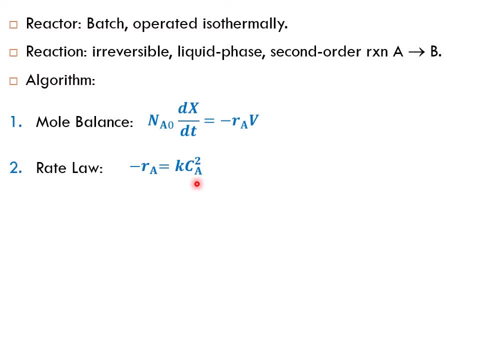 also a variable. so that means we need to provide an equation for c? a. so we go to the stoichiometry and we find an equation for c? a. c a equals n a over v. n a equals n a naught times 1 minus x and 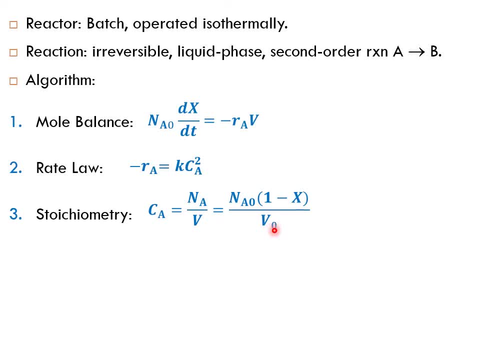 v equals v- naught, sorry, i forgot to put the not here- and therefore we can write the equation as: c a equals c a naught times 1 minus x. then comes the combined step and the combined step. we're going to combine all of the equations above into one equation, so we're going to substitute for c a using this equation. 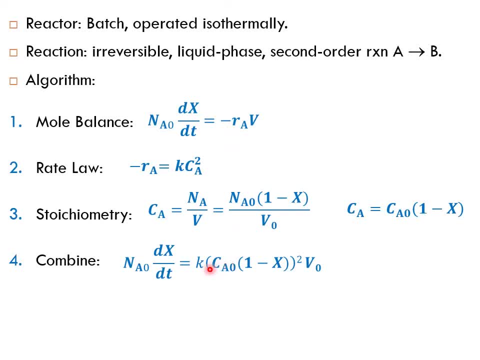 so for minus r a, we will have k. there we go k times: c a square, this is c a. so we got c a naught, 1 minus x, and it is squared. and then of course, v equals v naught and we have here an? a naught. all of this in the combined. 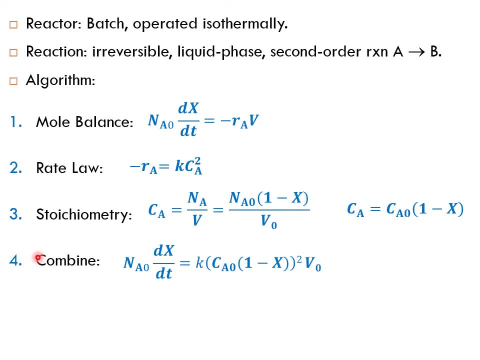 step and finally, we're going to evaluate. we're not going to evaluate the parameters now, but we're going to evaluate the equation. so let's rewrite this equation in such a way that we will integrate this function now. okay, so we need to integrate. you can either integrate. 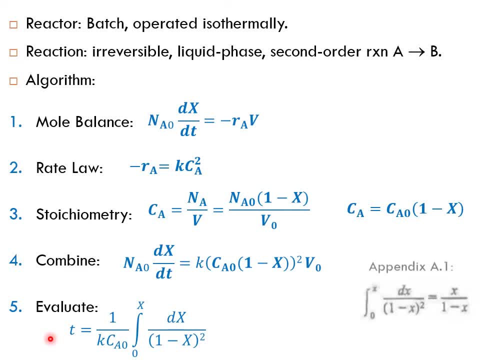 your knowledge and calculus, or you can go to the appendix, appendix a1, and you can find that the integration of this function is basically x over 1 minus x. okay, so therefore we'll have the time equals 1 over k divided by c, a naught times x, which is the conversion divided by 1 minus x. 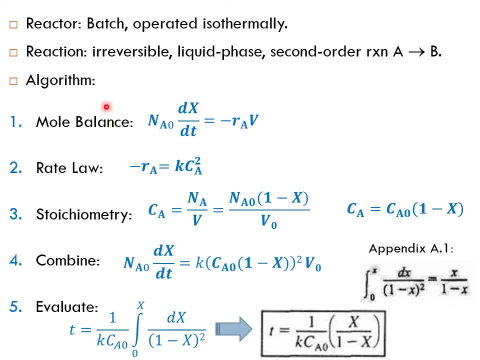 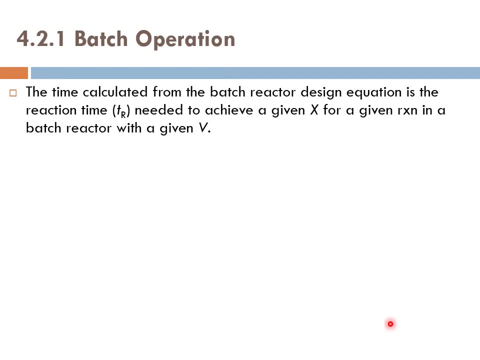 and this is the good example to show you how to use the five-step algorithm and design in designing a reactor. in this case it's a batch reactor. okay, so the time calculated from the batch reactor design equation is the reaction time tr needed to achieve a given conversion for a given reaction in a batch reactor with a given volume. it could be: 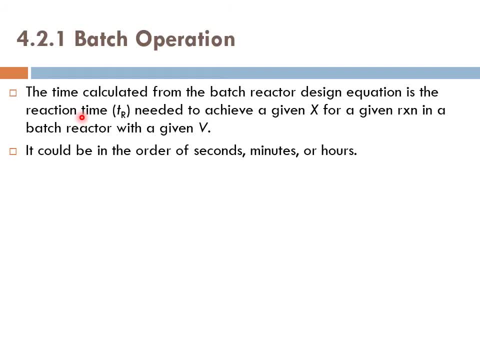 in the order of seconds, minutes or hours, depending on the rate of reaction. if the reaction was fast, then probably the reaction time is going to be in the order of seconds or minutes. if the reaction was so slow, then it's going to be in order of hours. the total cycle time. however, any batch 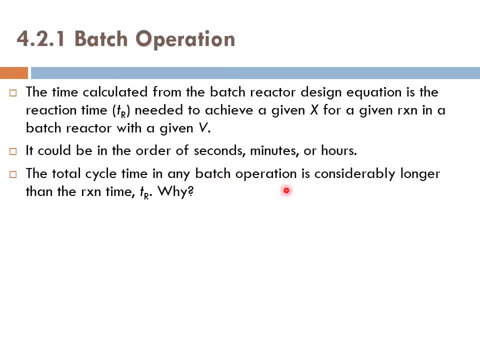 operation is considerably longer than the reaction time tr. why is that? that's because the total time to process a batch includes the time necessary to fill the reactor. you have to put all the reactions inside reactants inside the reactor and also you need to heat and or. 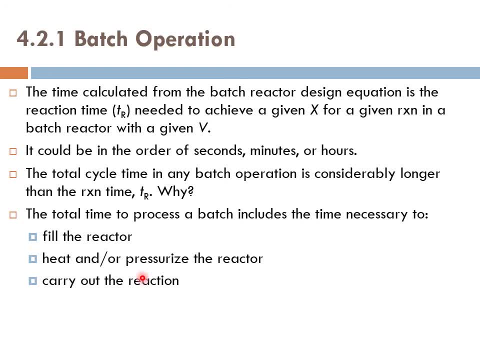 pressurize the reactor to the desired condition and then you carry out the reaction. and when you carry out the reaction you have to put all the reactants inside the reactor and also you need to you carry it out for a time that is known as the reaction time tr. then of course, after you finish, 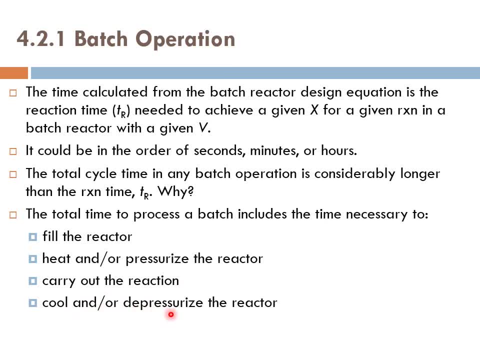 the reaction. you need to cool down or depressurize the reactor, remove all the products out and then clean the reactor between the batches. so you can see that only this step is known as tr. however, if you need a reaction time, you carry it out for a time that is known as the reaction time. 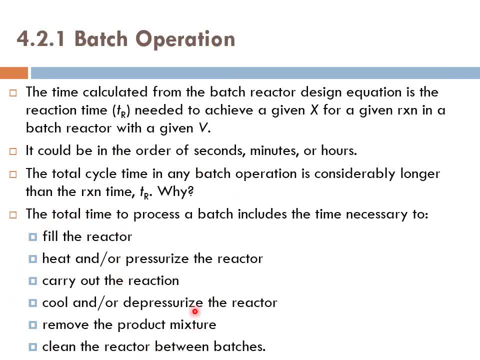 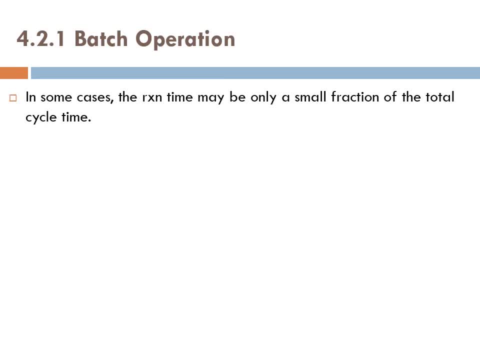 is the total time of the process. you need to sum up all the times required for each of these steps together. in some cases, the reaction time may be only a small fraction of the total cycle time. typical cycle times for a batch polymerization process vary from three to six hours, excluding the reaction time. the reaction time may vary between: 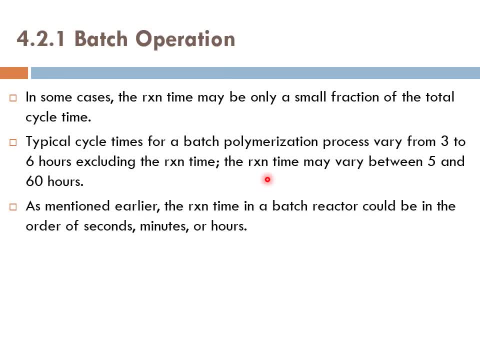 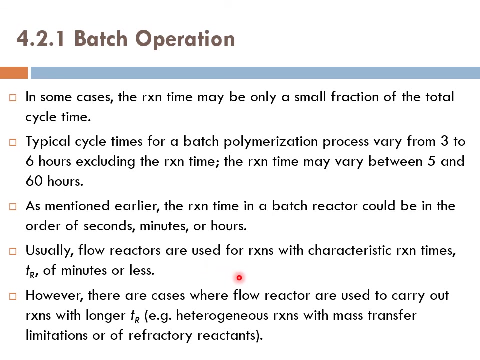 5 and 60 hours. as mentioned earlier, the reaction time in a batch reactor could be in the order of seconds, minutes or hours. usually, flow reactors are used for reactions with characteristic times TR of minutes or less. however, there are cases where flow reactors are used to carry out reactions with longer TR. 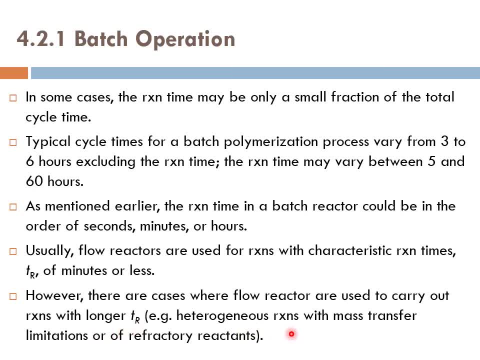 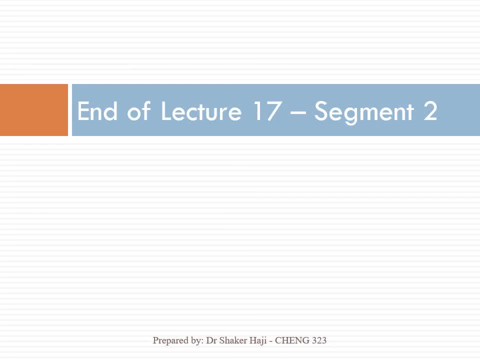 example, we have heterogeneous reactions with the mass transfer limitation or of refractory reactants. so with this we reach to the end of lecture 17, segment 2. we're gonna meet again to explain the last segment of lecture 17. see you then.